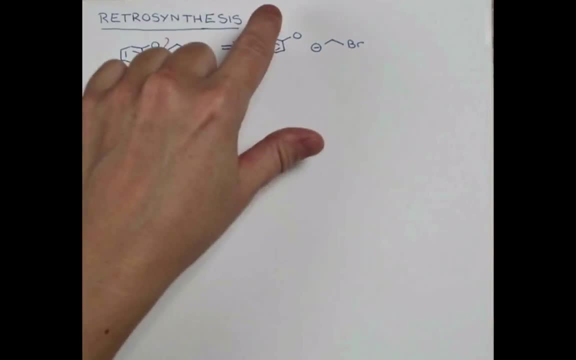 with a negative charge here. So now, if this is negative, well this would have to be positive. Now, this kind of polarity on these molecules which are synthons, these are idealized reagents to just show what would be a nucleophile and what would be an electrophile. They're going. 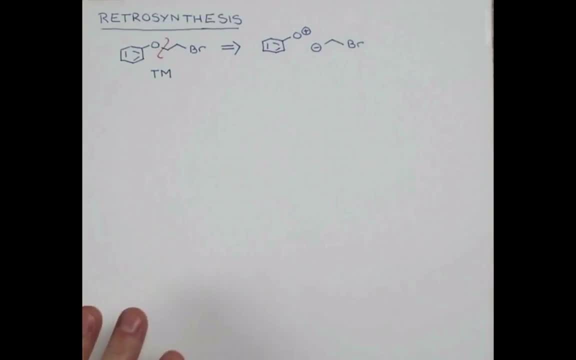 to correspond to an intermediate along the path. but they're not real reagents. But these aren't very good. Look at oxygen. We have a positive charge on it. We think of oxygen typically as a nucleophile. The lone pairs on oxygen attack things, And here we'd have to have some sort of grignard. 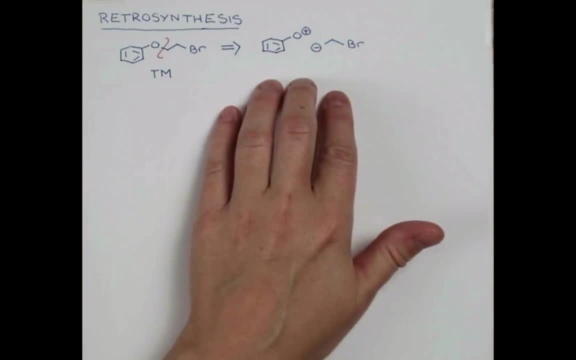 with another bromine in it. This is not the natural polarity that this type of reaction would take on. So if we did this and set this up as our synthons, you should notice that oxygen being positive and getting attacked. that doesn't really. 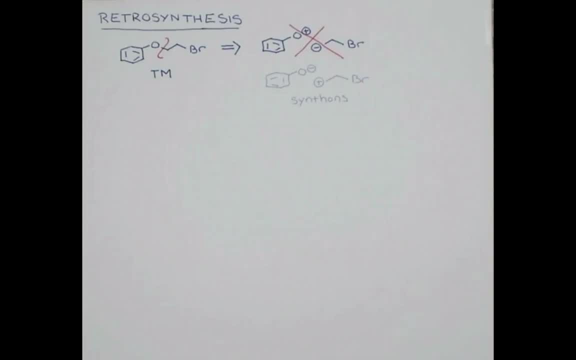 happen. Let's redraw them with the correct polarity. Here are our correctly drawn synthons. The oxygen has negative charge. This is natural. Oxygen tends to have negative charge And this more electropositive carbon has positive character in our synthons. 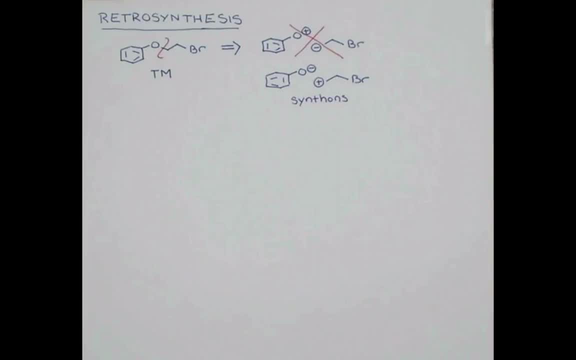 The nucleophilic partner. this one is going to be called our donor synthon. It donates the electrons And this one will be the acceptor. Alright, now I can't go to Sigma Aldrich and find synthons. I just can't buy these. 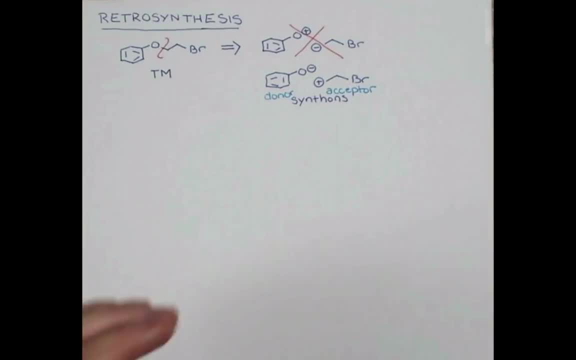 things. I need to buy reagents. So what could this translate to? Well, this one is pretty easy. It has an O minus, but we know that phenols are pretty readily available, maybe from our electrophilic aromatic substitution chapters. 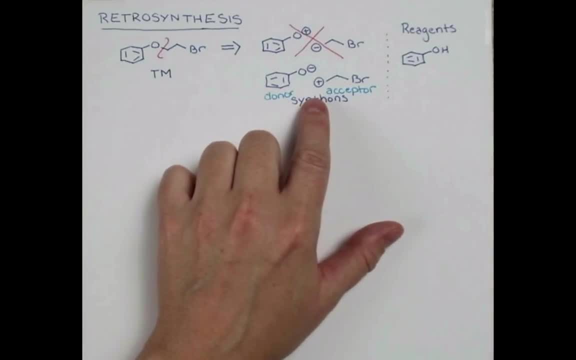 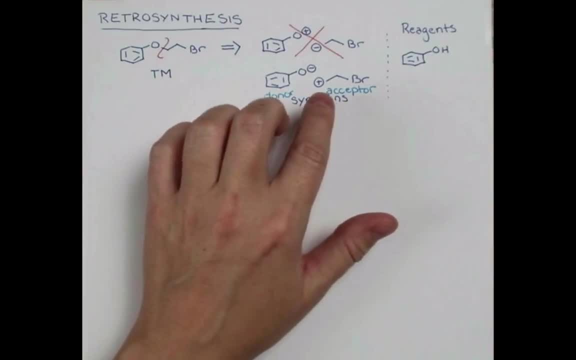 So to have carbon have positive character, something that's inductively electron withdrawing will give that positive character And if the leading group leaves, it forms a carbocation. Of course this is a primary, But remember this is a synthon. 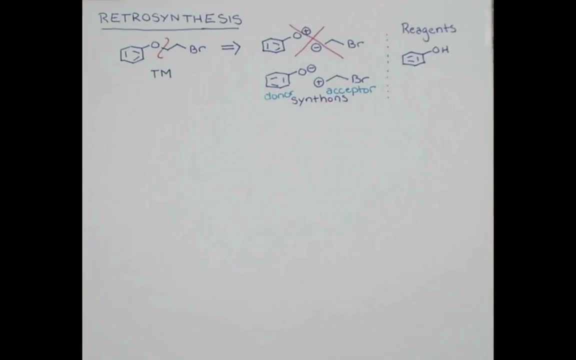 This is just a device to help us think about what we need to put together. So maybe we could have just a bromide on this side as well, And one of the bromides will leave in our reaction. Our reagent will be this. 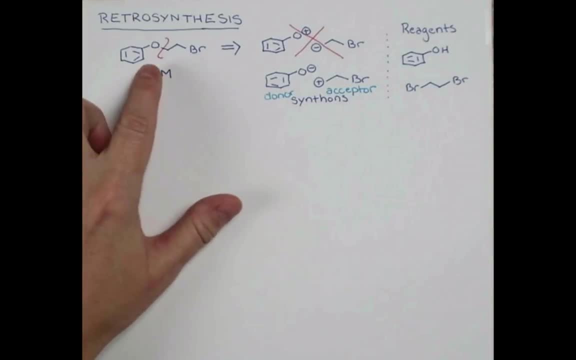 1,2-dibromoethane. here In this example, I told you we wanted to cleave this bond. This is a pretty good rule: cleaving next to a heteroatom. So if we can cut a bond and think, 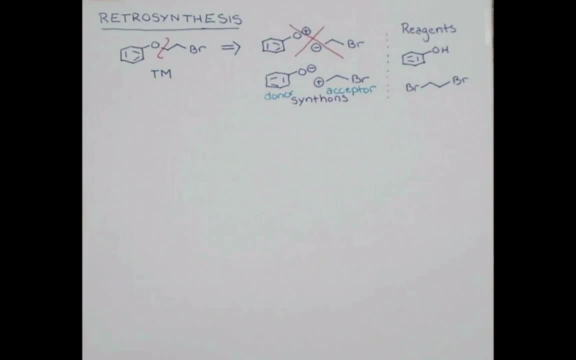 about a reasonable reaction that we know from all of our organic chemistry to make this bond in ether linkage. that's great, But there are a couple places that are next to these heteroatoms that I didn't cleave and I want to show you why, before we move on to lots of reactions and 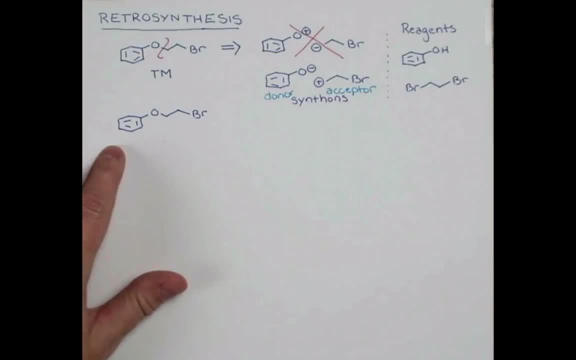 examples: Here's our target molecule redrawn. Now I'm going to draw some other disconnections. We'll cleave on the left side of the ether and call this A, and then we'll disconnect adjacent to the bromide and call that B. Okay, neither of these is a very good disconnection, so why not? 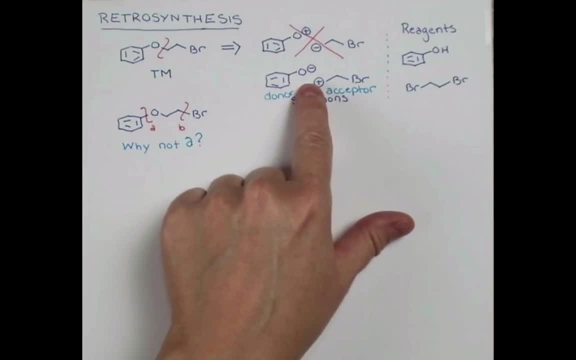 With A, if we're capitalizing on the natural polarity of oxygen to be negative and a nucleophile, we're going to end up with an aryl cation. Let's draw our synthons Now. this aryl cation might look familiar from the diazonium reaction. 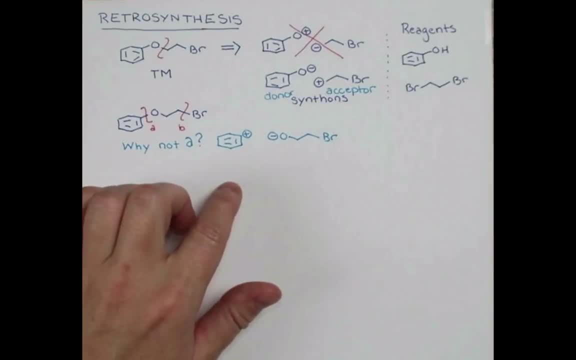 so these can be formed, but they're really high energy and this is kind of a difficult reaction. This isn't the natural polarity of an aromatic ring. Now, if we had electron withdrawing groups on here, we could think of maybe a nucleophilic aromatic substitution involving a positively 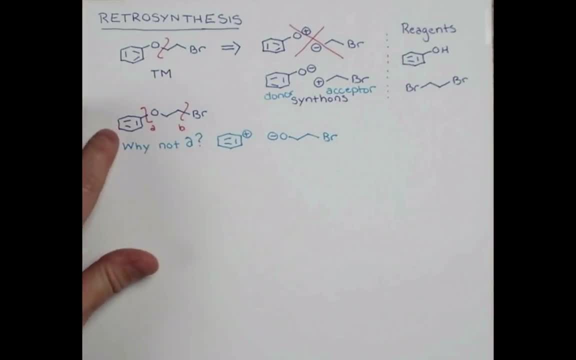 charged area on an aromatic ring. but for this unsubstituted reaction we're going to have to do a nucleophilic aromatic substitution. That doesn't really apply. so there's no reason we'd do nucleophilic aromatic substitution. Doing a diazonium reaction is not as reliable as the 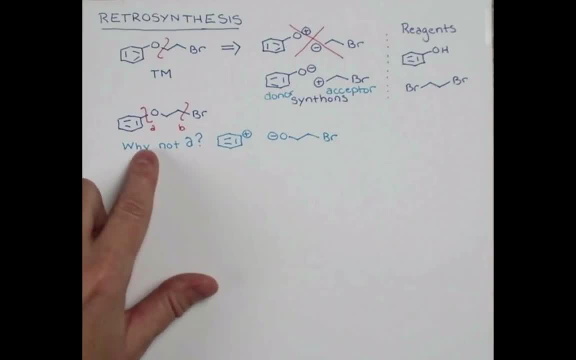 Williamson etherification. so that's why A would not be our best disconnection. Okay, why not B? All right, so we just broke the bond. We haven't put on our polarities yet, but bromine usually has a negative charge. Br- is a good leaving group, a good nucleophile, so let's assign that polarity to. this synthon: Br- is a good leaving group, a good nucleophile, so let's assign that polarity to this synthon. Br- is a good leaving group, a good nucleophile, so let's assign that polarity to this synthon. 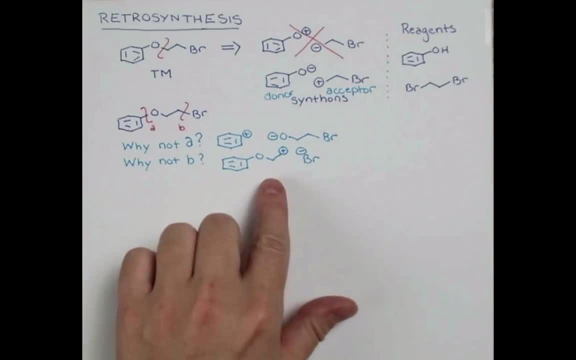 Now we need a positive charge here, Okay, well, we saw we could do that Carbon is an electropositive atom and we came up with something like this. So why would we put a leaving group on a carbon just to replace it with another group? That doesn't simplify our synthesis at all. We 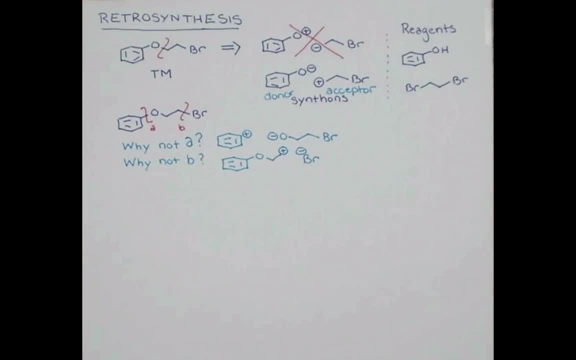 already need to have all of this built up if we're adding on the bromine in the last step. so this doesn't make sense either. So our best disconnection is cleaving here to the right of the heteroatom and using the negative charge of oxygen in, perhaps, a Williamson ether synthesis. 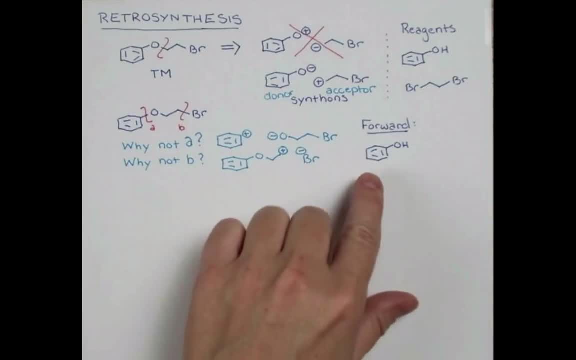 Now we can draw a forward synthesis, Beginning with phenol. we can treat this with base, perhaps sodium hydride, and then add in our bromide, and this should give our target molecule. This analysis is going to work for sulfur too, so let's make this compound very similar to this one. 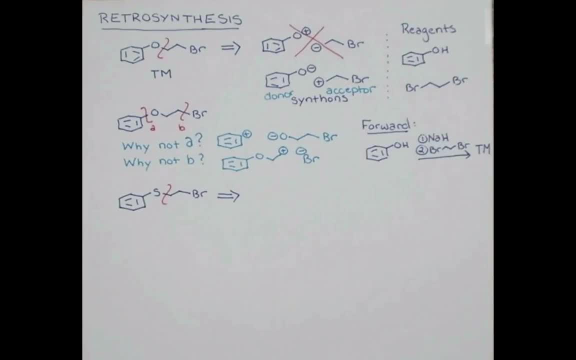 We'll disconnect in the same place. and now I want to introduce a little terminology that we can write above the arrow. We can tell what bond we're cleaving, and here it's a carbon sulfur bond. so we write Cs like this Up. here. we can write Co, and sometimes we'll put the functional group name. 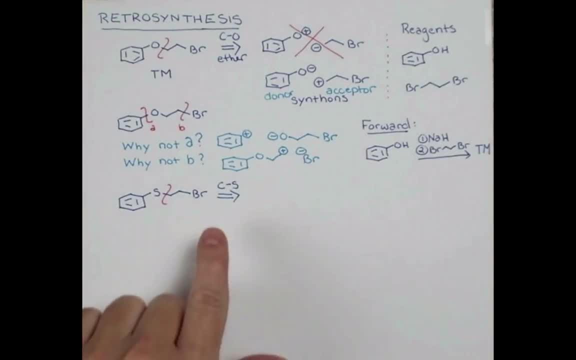 as well. So Co and making an ether Cs, I could put thioether Sulfur is a good nucleophile in SN2 reactions, so that has the negative charge. We have the same bromide, and so let's show what. 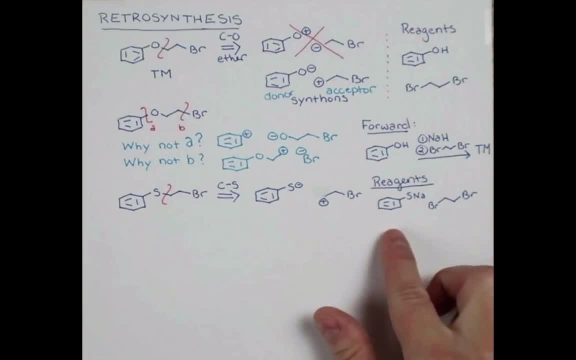 reagents we might be able to use. These are both carbon sulfide bonds and these are carbon sulfide bonds For both commercially available compounds. we have the sodium salt of this thiophenol here, so this is an S-NA+. You can buy it as the salt from Sigma-Aldrich and it's useful. 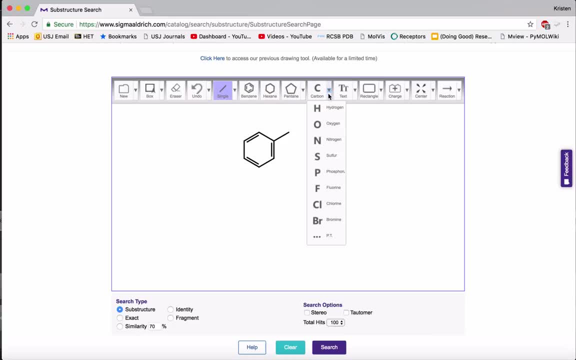 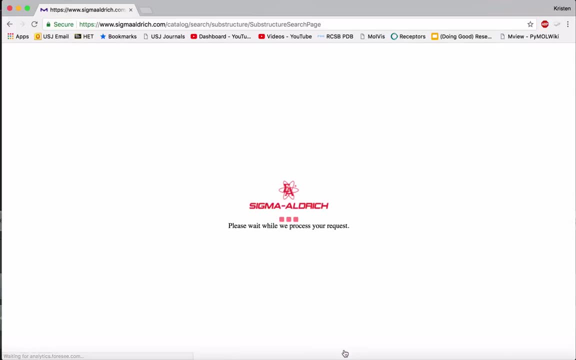 There's a webpage you can go to the Sigma-Aldrich structure search which allows you to put in a structure and search for similar structures or that exact structure and see if you've gotten your synthesis back to commercially available compounds. Let's try and explain this. 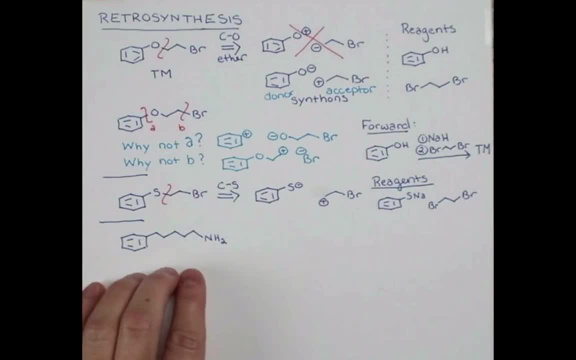 Let's take an example with an amine and see if it'll work out the same. Although this is a pretty simple looking molecule, it is not commercially available, And so you might think, oh, I could probably substitute this amine for maybe a leaving group, maybe a halogen, So that would be a 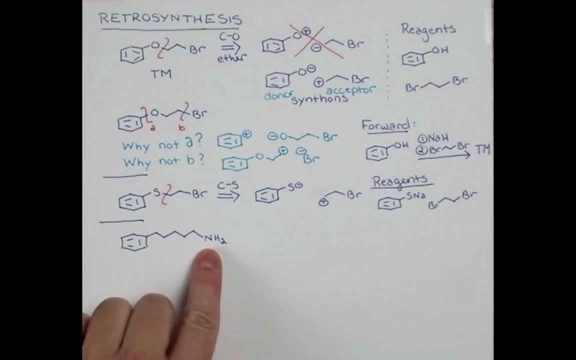 different transformation. We're not really breaking a bond, we're just changing a functional group. So let's introduce another bit of terminology. We're going to write Fg over the arrow to show this would be a functional group conversion. The hormone that is corresponding bromide is commercially available.